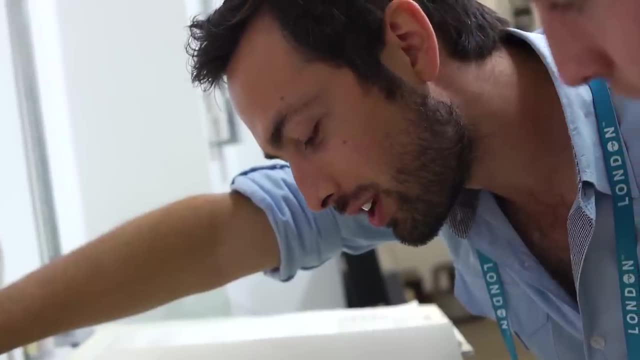 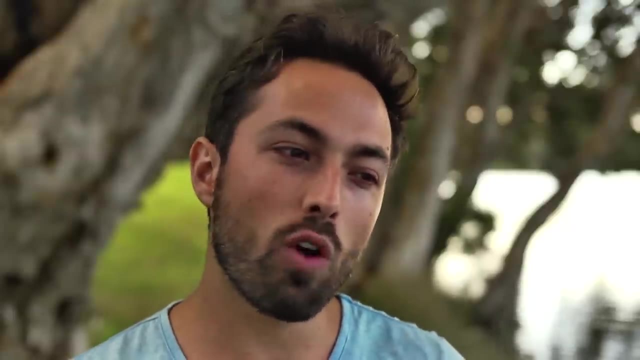 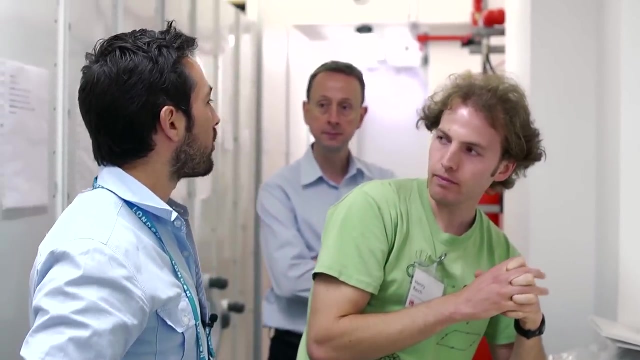 the shadow itself was divided by six Similar parallel fringes of smaller dimensions. Wow, This is an experiment so simple that you could make it at home, and yet so fiddly that I have never seen it before done with sunlight. I was thinking about doing it in a box, like a fridge box. 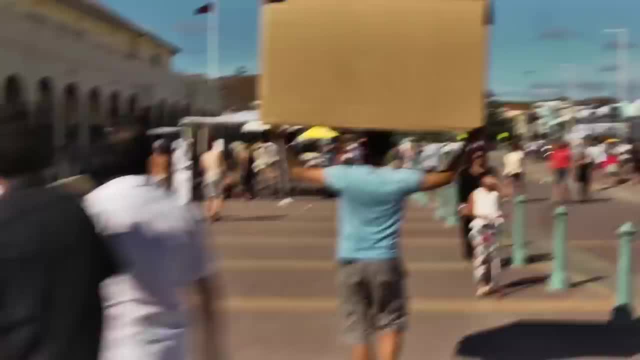 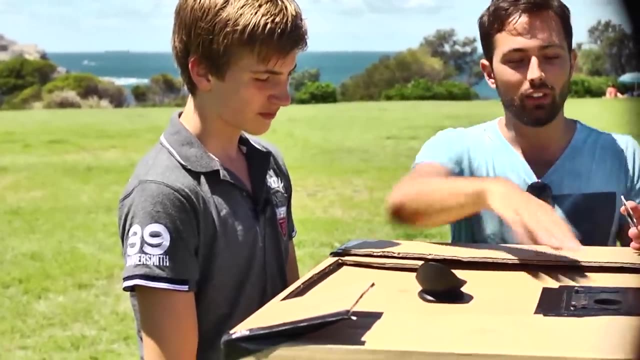 And you could take it out on the street. Taking it out on the street, Could I possibly interview you guys for about a minute? We're doing a science experiment. What I have here is an empty box And this is a little eyepiece where we can look in, and this is a hole. 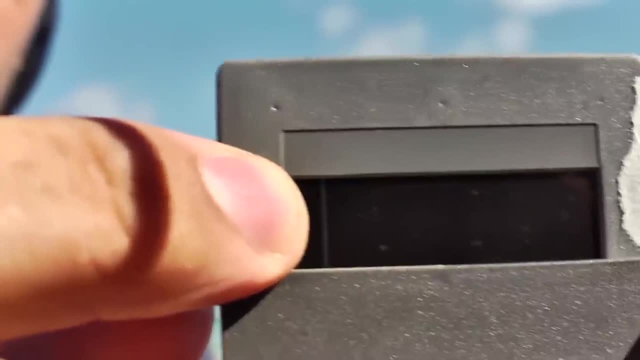 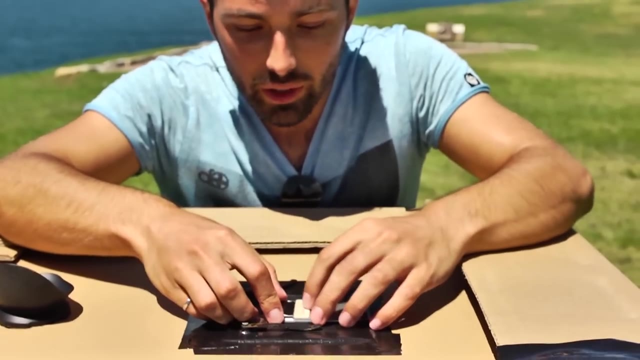 We're going to place this slide above that hole and if you look closely, you'll see that there's two openings, Very narrow openings, side by side. It's a double slit. Now, before we have a look, we need to tilt it towards the sun a little bit. 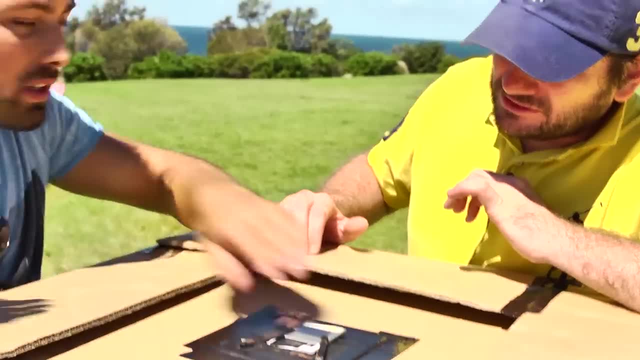 so we want the sun to hit this double slit directly. What are we going to see on the bottom of the box? The obvious thing you think you're going to see is you're going to see two lines, Two lines on the bottom of the box. 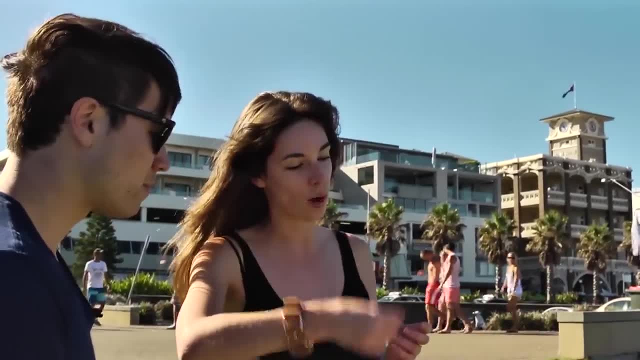 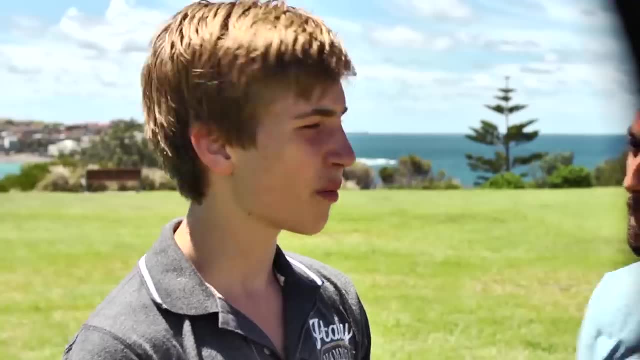 Two bright bands, Two little lines- Yeah, I think it'll be one line instead of two. I can expect to see the whole box lit up, A light discolour of some sort, A bunch of colours, Probably, yeah, Rainbow, different colours. 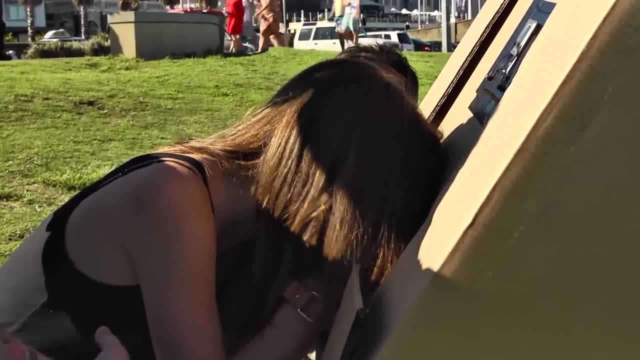 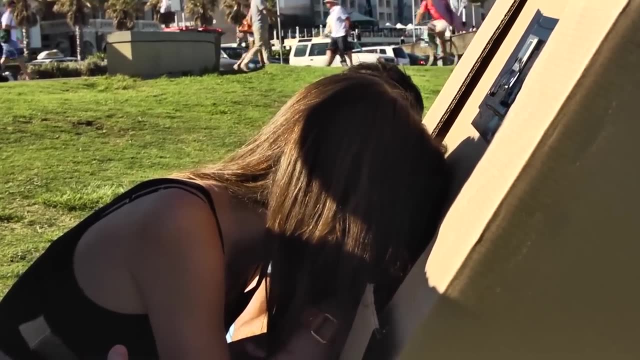 There have a look. You expected to see kind of one line. Is that what you see? No, I see dots. How many It's one circle? Well, there's one in the middle, strongest, two either side. The two on the outside are multi-coloured. 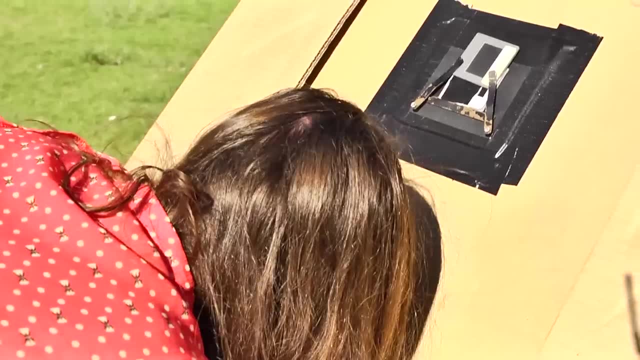 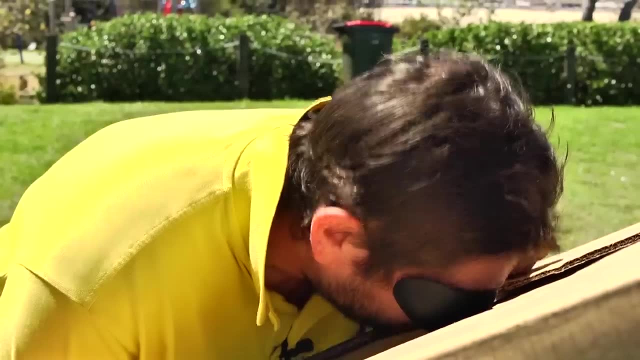 and the one in the middle is just white. It's kind of a rainbow, The rainbow of colour as well. Quite a few colours and lots of little dots. Like there are more dots appearing. I think I can even see more dots spreading along. 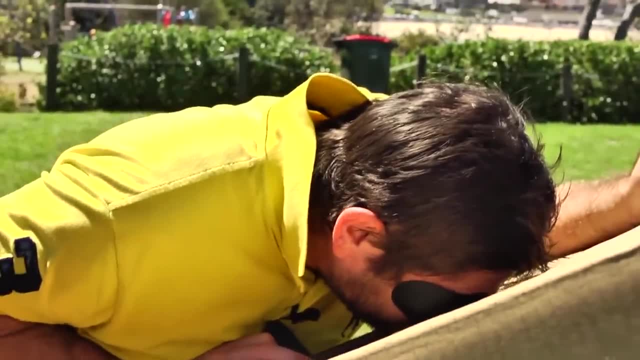 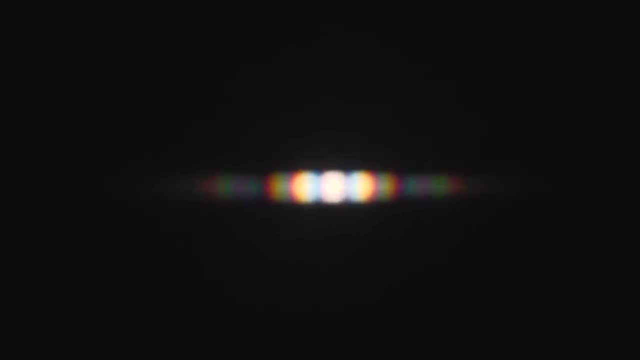 Yeah, that's amazing. Yeah, I can see tons of dots- now, Not tons, but I can see dots spreading across that way, Either side. Yeah, definitely, Isn't that amazing? Yeah, that's incredible. And that's just nothing else apart from. 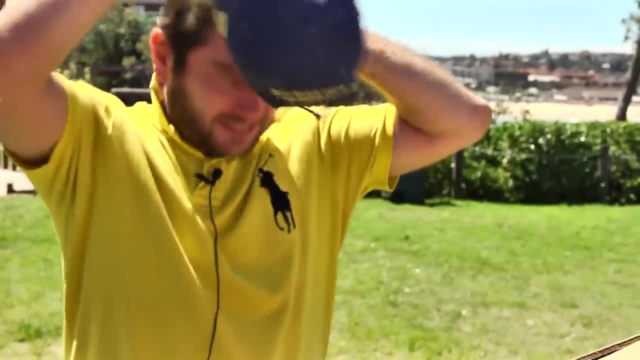 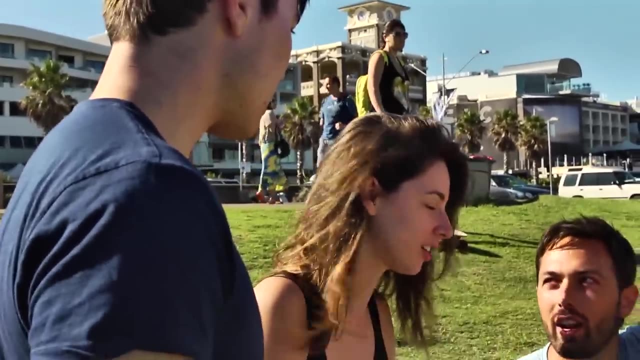 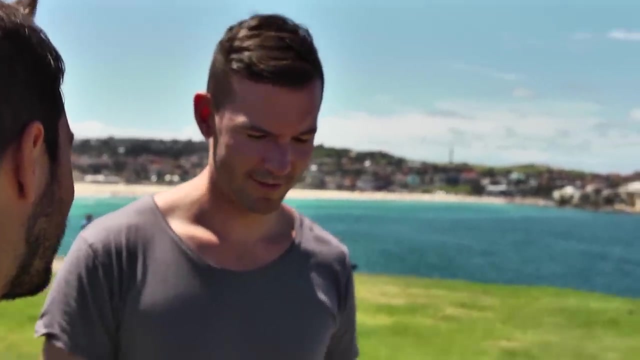 Two slits, Two slits. That's incredible, But all we're doing is we're putting a light through two very narrow slits side by side. So how does this make any sense? There's some kind of principle involved there that the average person is not familiar with. 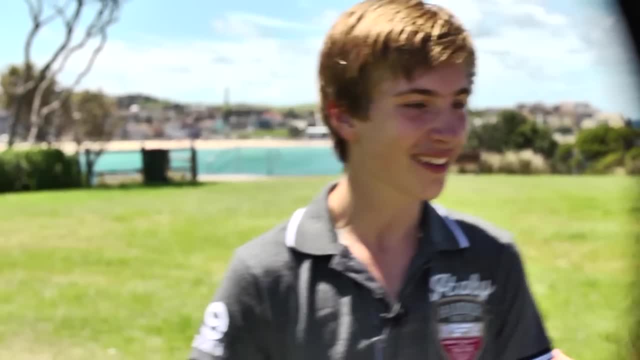 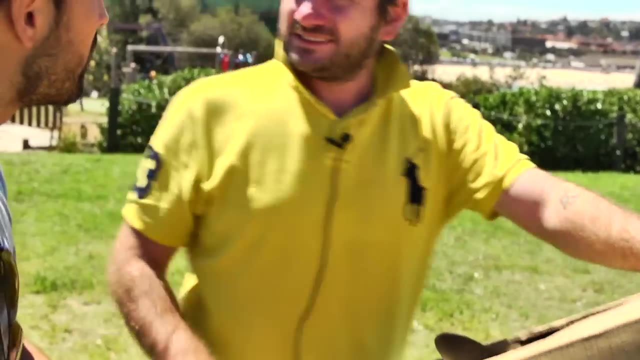 That's the only explanation. I'm really confused by it, but I'd like to find out why People were debating. is light a wave or is it made of particles? So what causes that? Well, if light were behaving as particles, 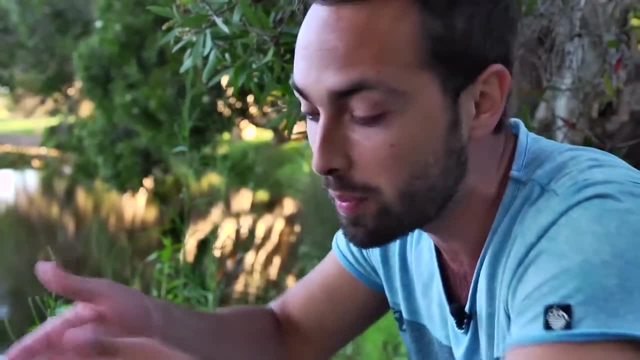 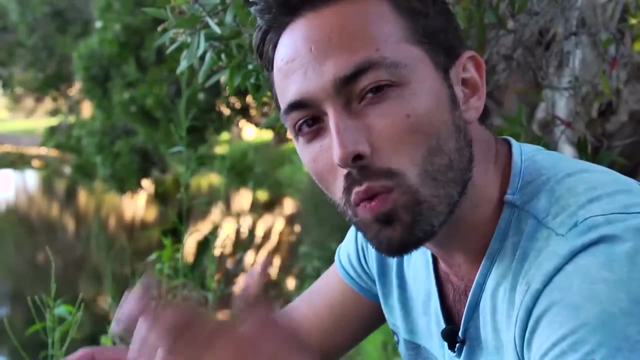 you would expect them to go through each slit and just produce a bright spot underneath, So we would see two bright spots on the bottom of the box. But if light's behaving as waves, then the wave from one slit can interact with the waves from the other slit. 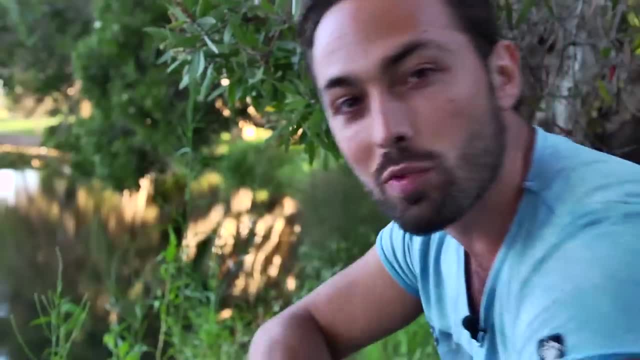 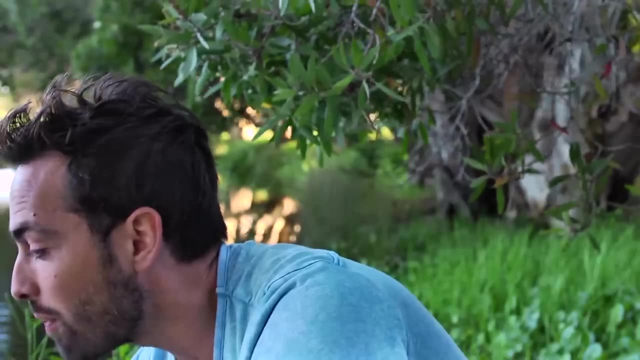 I've got a demonstration here on a little pond where we can see this. with water waves I have two sources of ripples which are basically like the two slits. When I create ripples with a single source, they travel out with circular wave fronts. 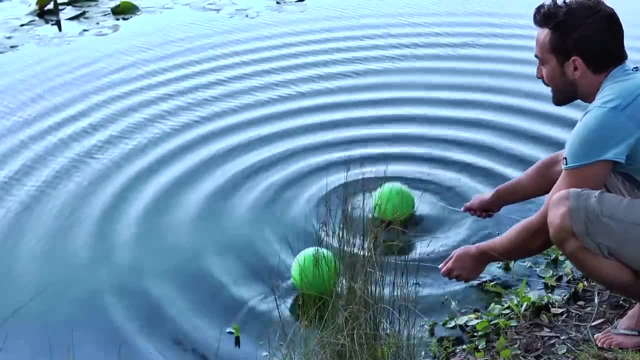 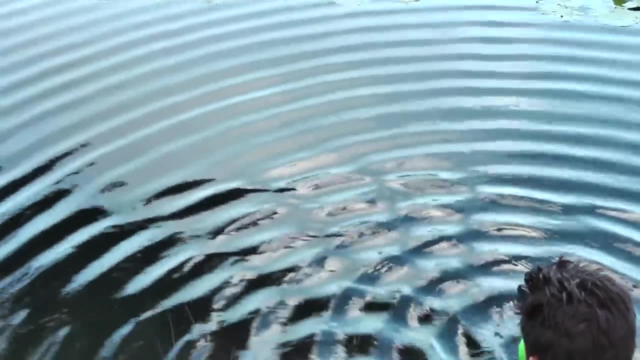 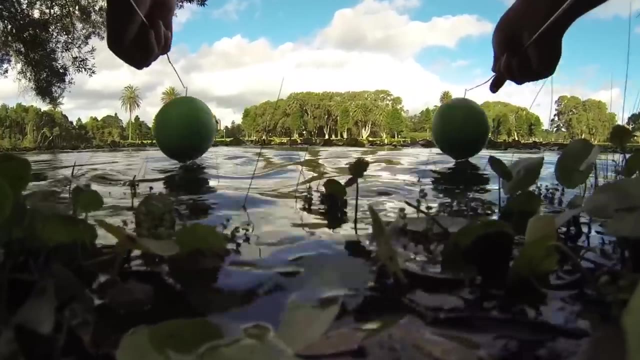 Nothing particularly surprising there, But if I add a second source of ripples, then we start getting an interesting pattern. This pattern is created by the ripples from the two sources interacting with each other Where they meet up: peaks with peaks and troughs with troughs. 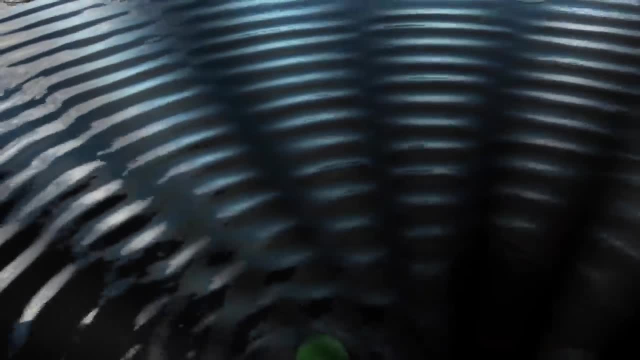 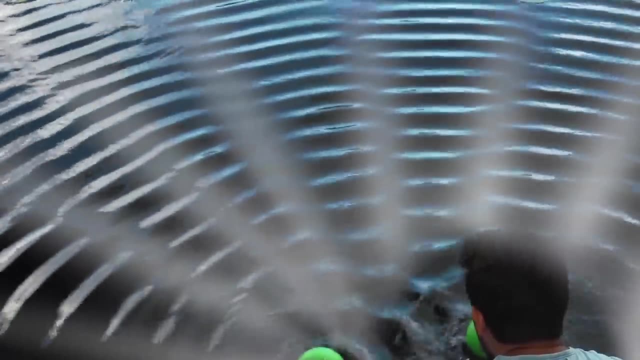 the amplitude of the wave is increased. That's what we call constructive interference. But if the peak from one wave meets up with the trough from the other, then we get destructive interference and there's basically no wave there. And this is exactly what was happening with the light. 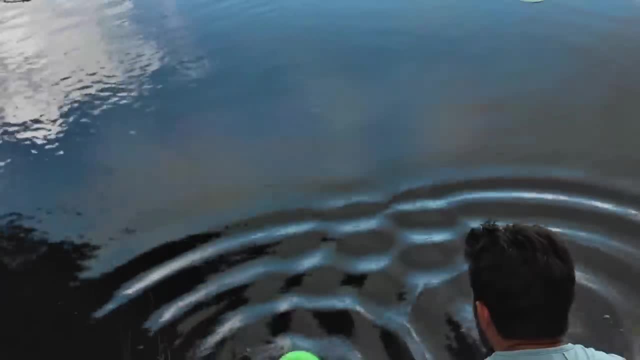 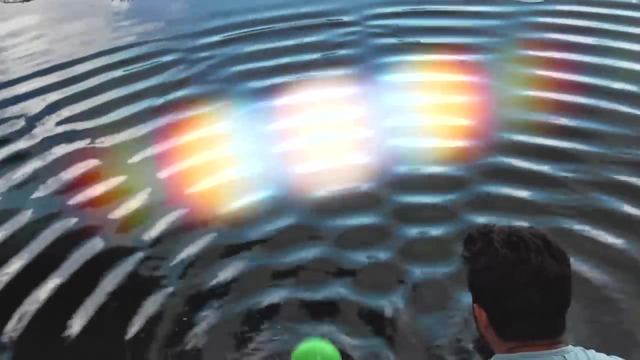 When the light from one slit met up peaks with peaks and troughs with troughs, they constructively interfered and produced a bright spot. But if the trough from the wave from one slit met up with the peak of the wave from the other slit, 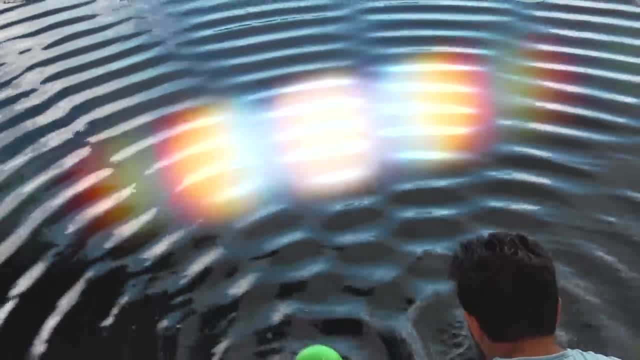 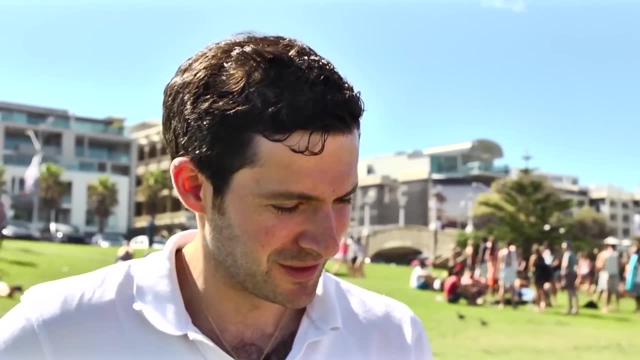 they would destructively interfere and you wouldn't see any light there. It's light cancelling itself out. This is basically the same as having two drops of water fall in a swimming pool. That's right, Exactly the same pattern. And then they go and overlap. 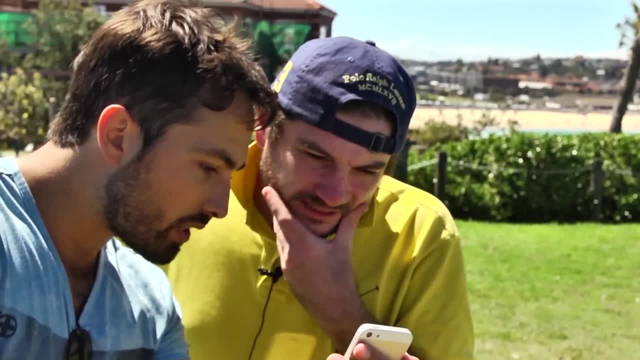 As this ripple overlaps with those ripples down the bottom, you get a series of. you get a bright spot and then a dark spot, and then a bright spot, and then a dark spot, and then a bright spot. Now there's a slight complication. 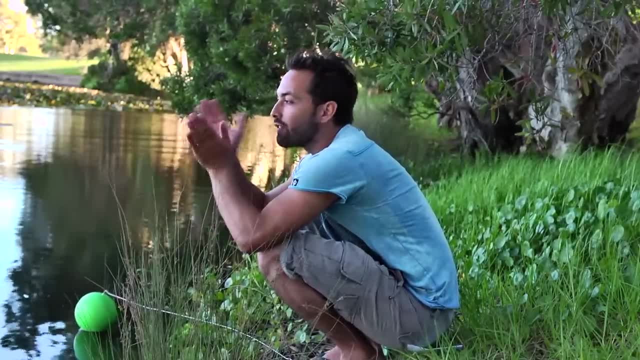 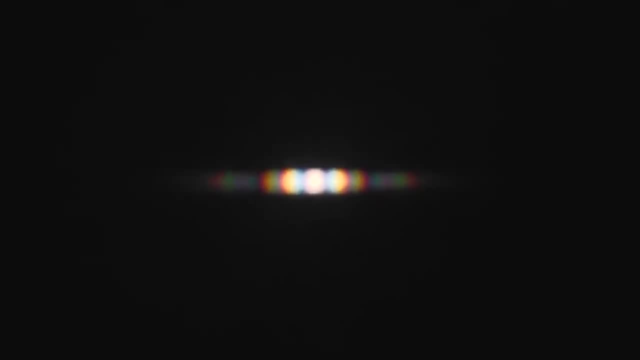 which is that sunlight is composed of many different colours and they have different wavelengths, So obviously they're going to meet up at slightly different points And that's what caused the rainbowing effects as we go further from the central maximum. You saw, the ones to the right were slightly coloured.